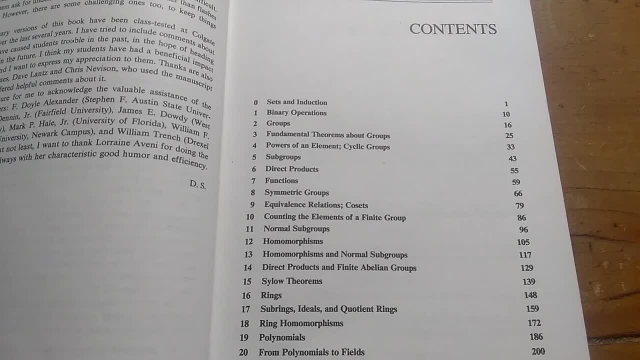 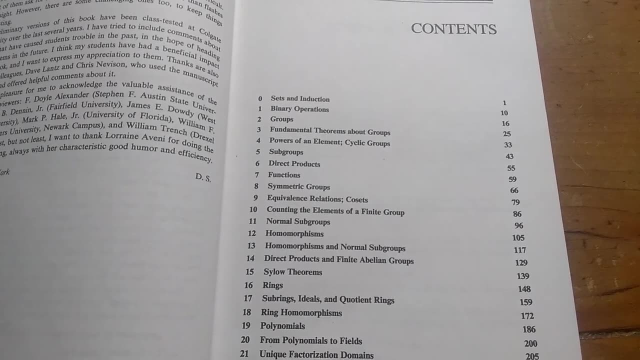 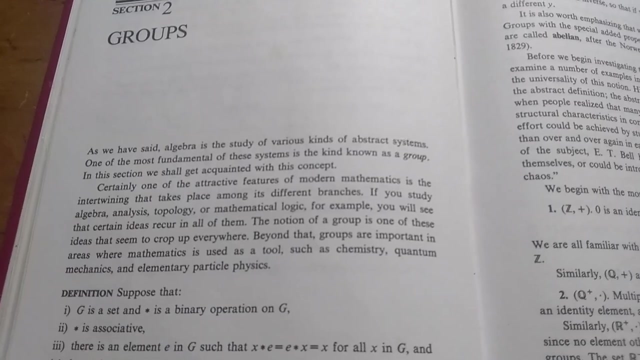 compared to other books. In other words, this is a very, very beginner friendly book. So what do I mean by beginner friendly other than the order of the topics? Well, let's take a look further inside. So the way the book is written is such that it's very easy to read. So it is very, very easy to read this 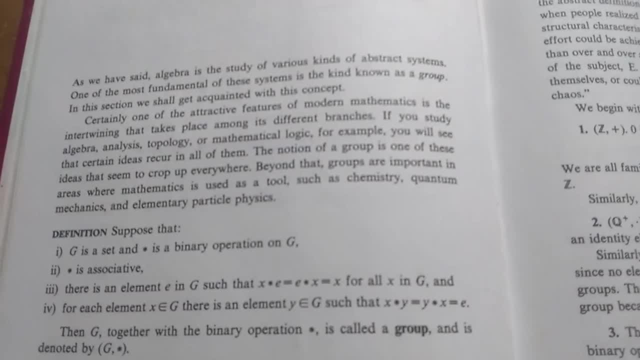 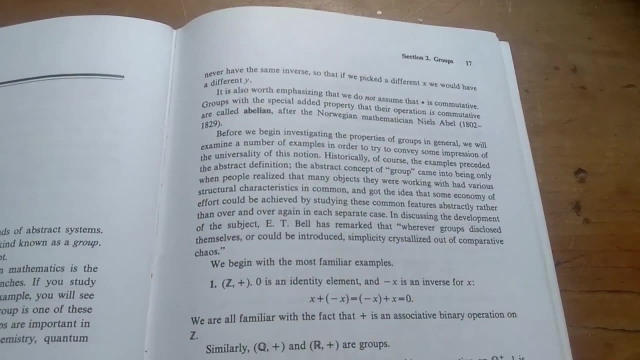 book. It might not seem that way if you're just new to abstract algebra, but trust me, compared to other books, this book is probably the easiest book to read. I'm not going to go too far on abstract algebra. 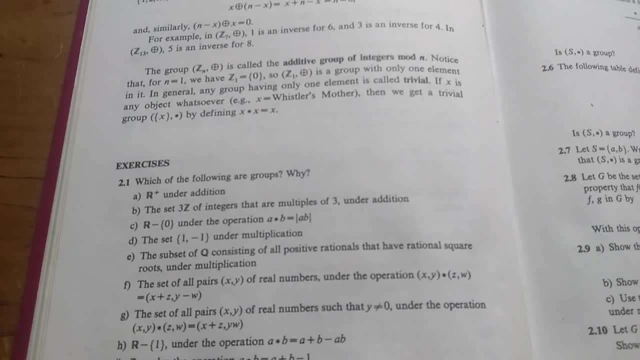 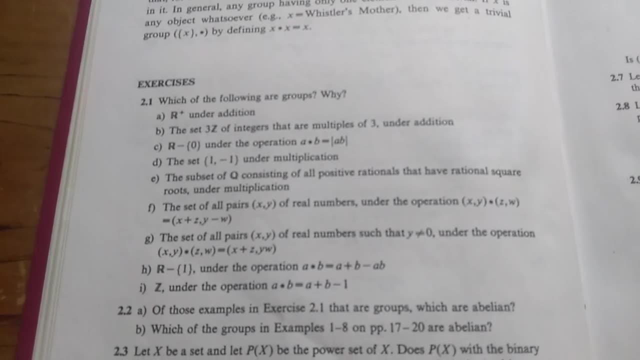 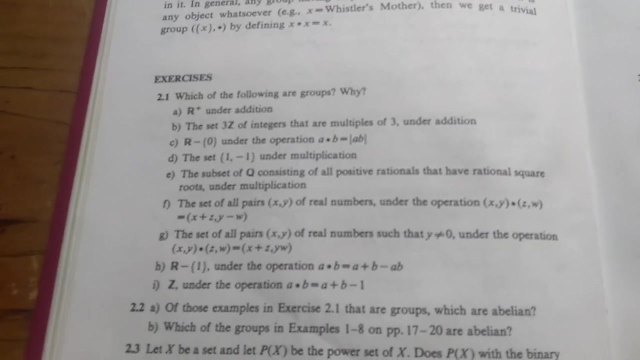 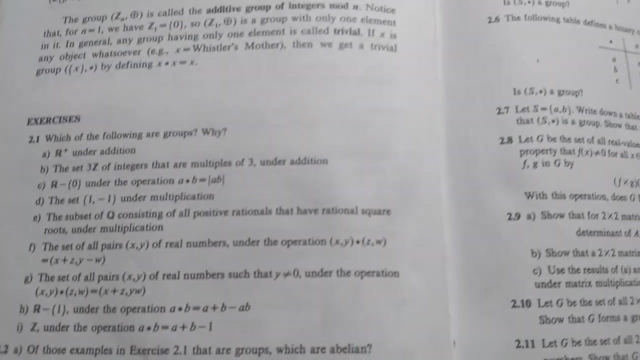 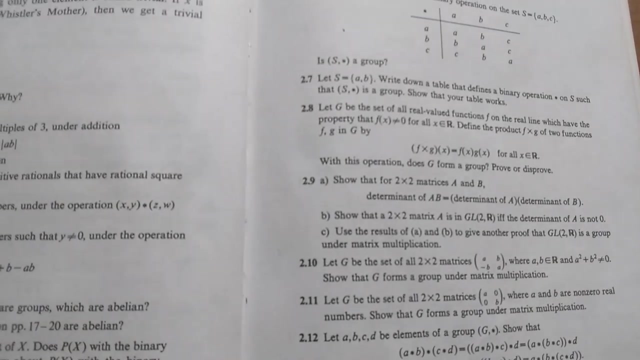 Another thing that makes this book really special is the level of difficulty of the problems. So the exercises at the end of each section are just the right level. Some of them are pretty easy. So they're like feel good problems, because you will feel good when you figure them out. And some of them are a little bit harder. So if you read the book and you really learn the material, in theory, you should be able to do most, if not all, of the problems. So it's a nice book if you're a completionist. If you feel 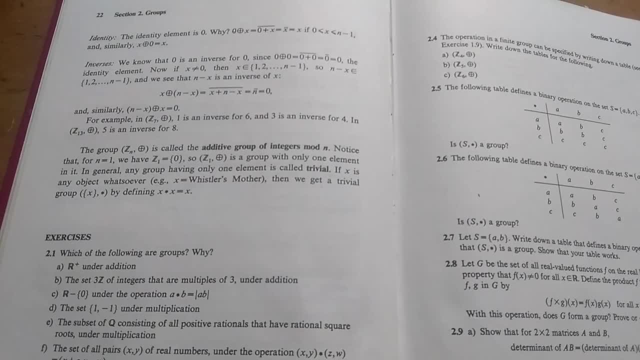 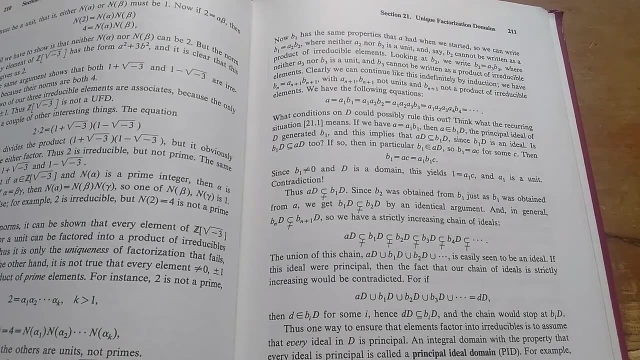 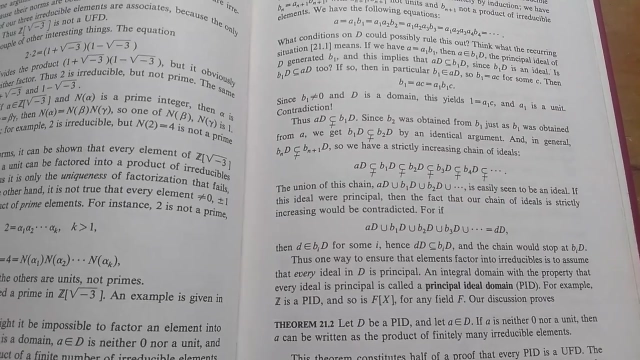 like you should do every single problem in the book, this is a really, really, really good book to try to attempt to do that. So what is the downside to this book? Well, I think the most negative thing about this book is the content, the amount of content. I'd wish that Seracino had 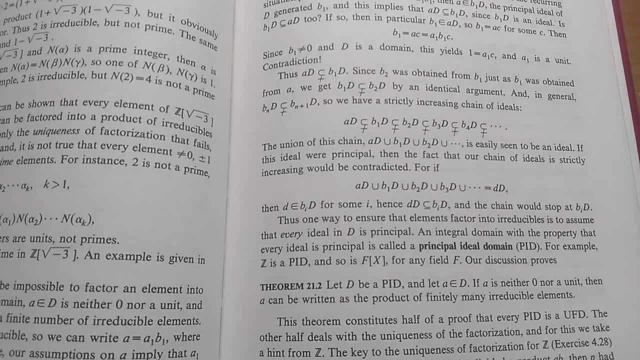 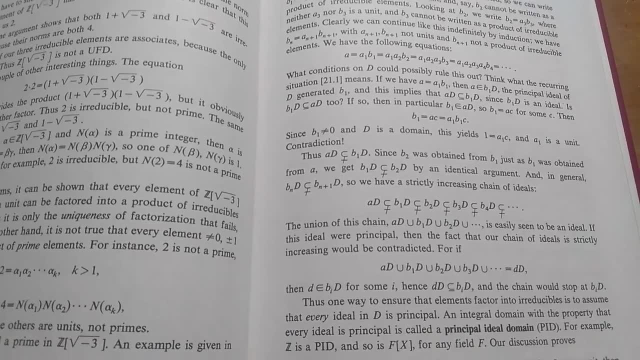 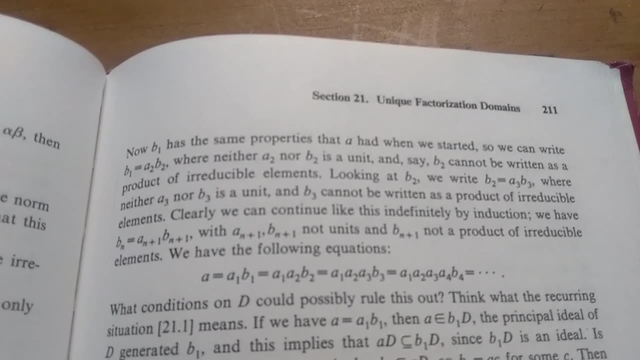 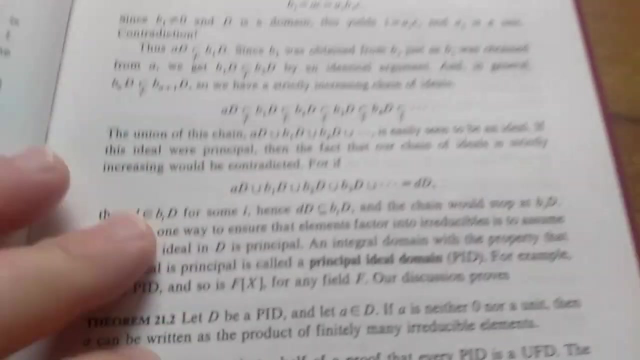 added more content to the book, but it's not really such a negative because if you actually make it through this book and you learn everything in this book, then you will know quite a bit of abstract algebra. For example, this is the last section in the book, I believe, section 21. It's on unique factorization domains, otherwise known as UFDs. So he does mention PIDs here at the end, principal ideal domains, but let's turn the page so we have some more stuff here. He talks about a Euclidean domain.